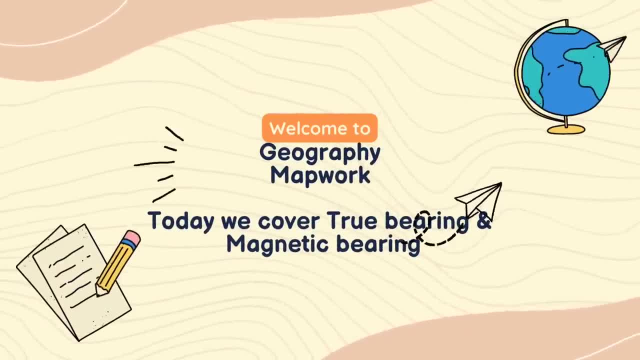 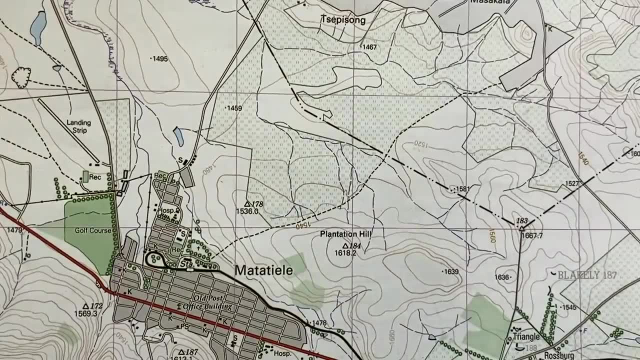 Hi Geographers and welcome to yet another tutorial video for Geography. In this video I'm covering True Bearing and Magnetic Bearing. So I'm going to try first to cover True Bearing and do Magnetic Bearing after calculating or finding the True Bearing. So let's get. 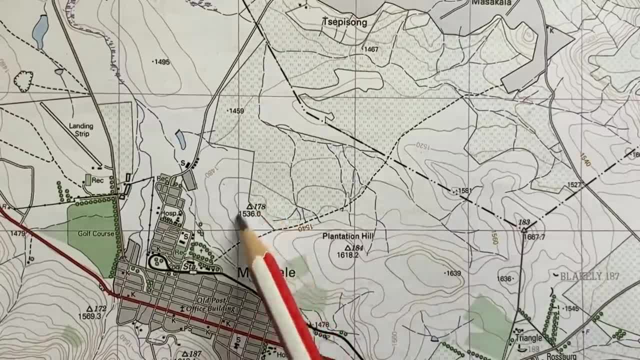 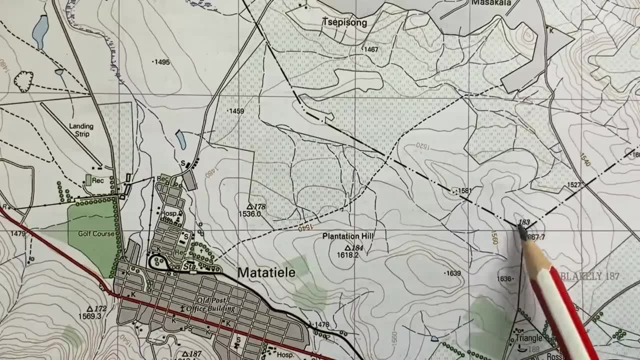 to it. So say you were asked to find the True Bearing from trickbacon178 over here to trickbacon183 over here. The first thing you need to note is the word from and to, and when you start, that's where you're gonna, that's where you're gonna put your true notes. So 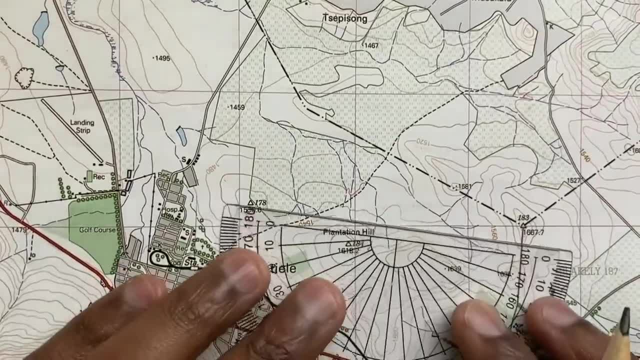 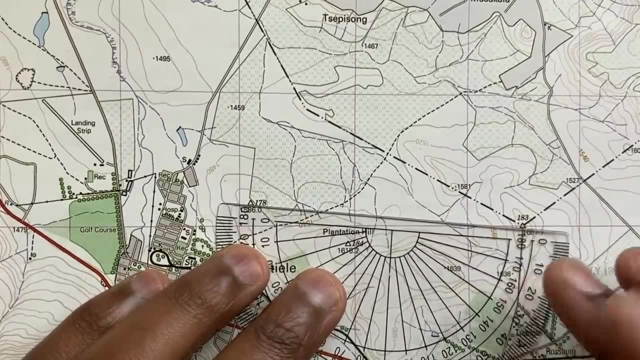 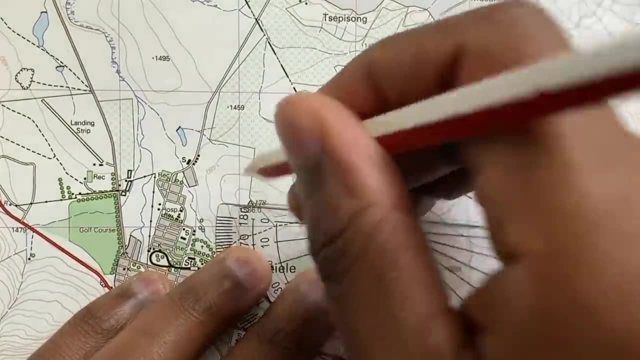 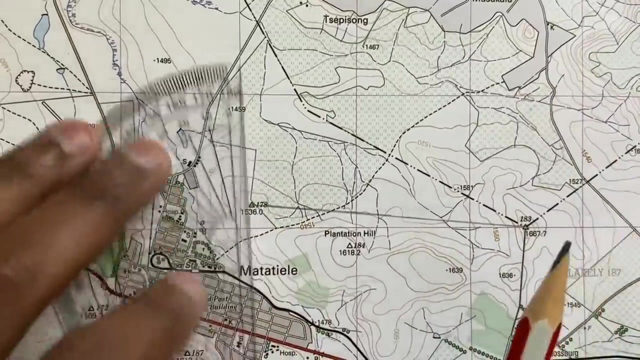 let's work this out. So first thing you need to do is join the two, The two trickbacons, with a straight line, And then our question says from 178.. So from here, that's where we'll put our, our true note. 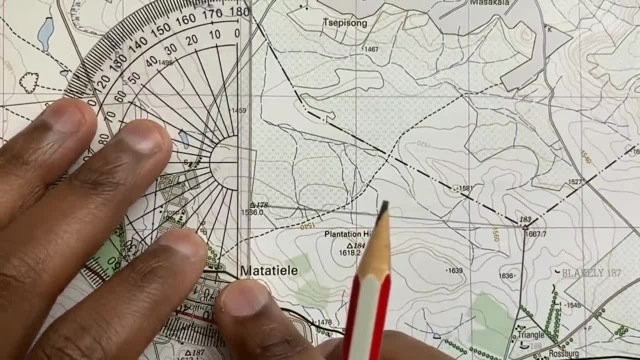 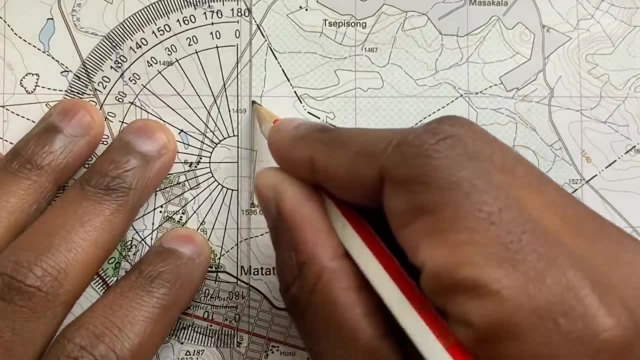 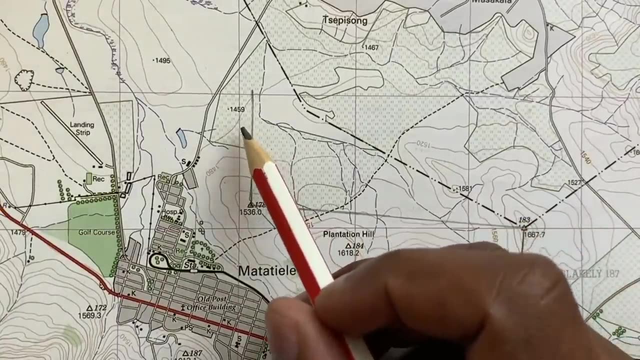 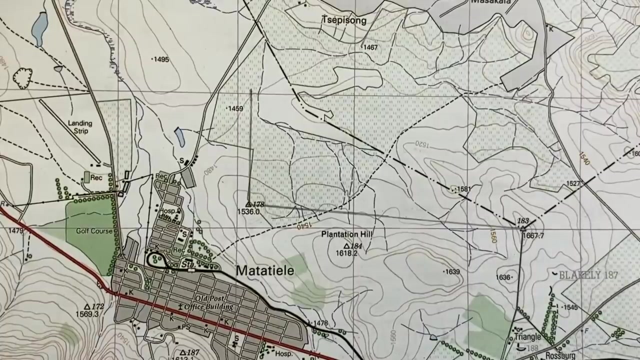 So your true note needs to be parallel to your longitudinal line over there, And you should start right in the middle of the trickbacon Over Over there, like that. The reason for your true note to be parallel to the longitude line is for you to be able to precisely and accurately measure the true note as accurate. 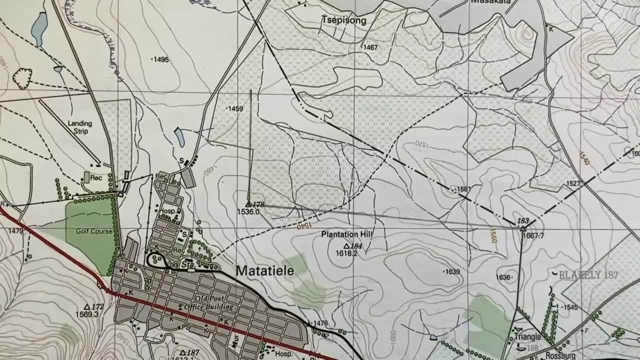 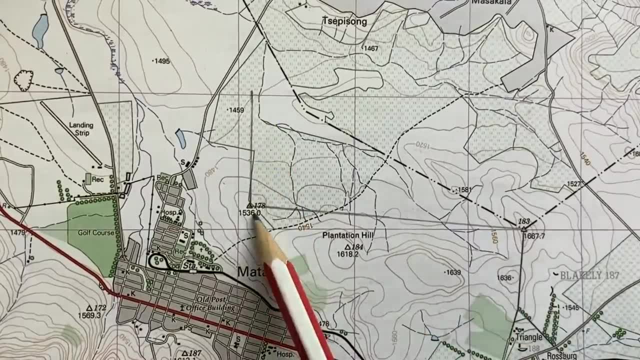 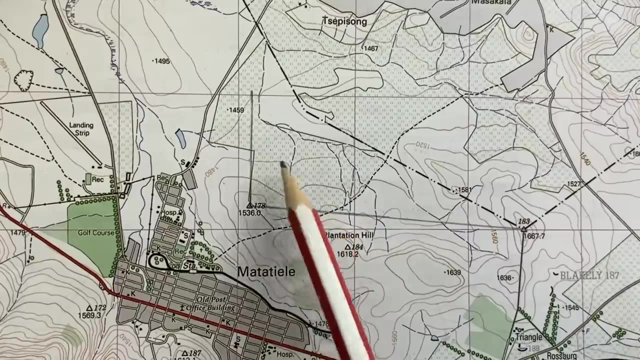 as possible. So what you need to do after doing here- because you have your true note and your line joining the two beacons, which is from 178. To 183- is just to measure the angle between the true note and this line in a clockwise. 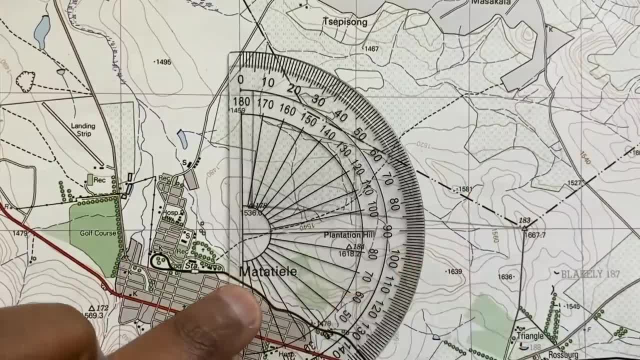 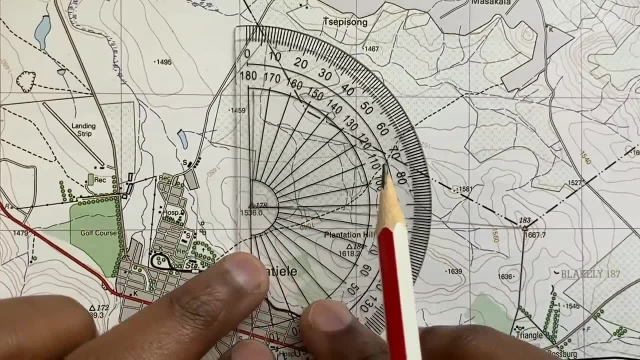 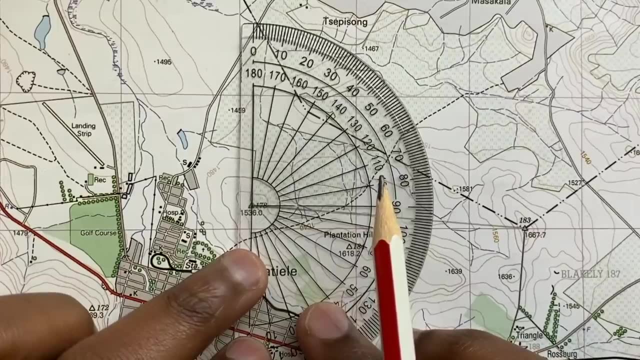 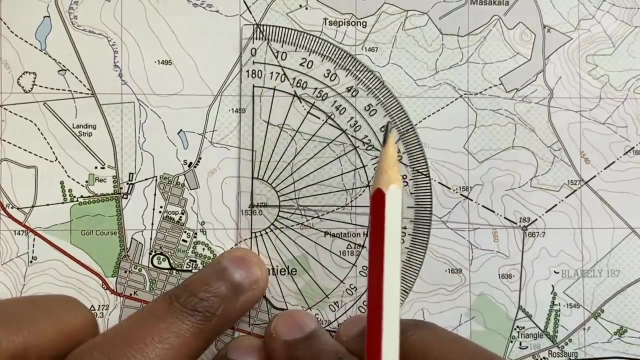 direction. So let's try to do that. So in so doing this T junction over here it needs to be directly in inside the trickbacon and your, your line, or this line Or this line of a protractor, over here it needs to be directly. 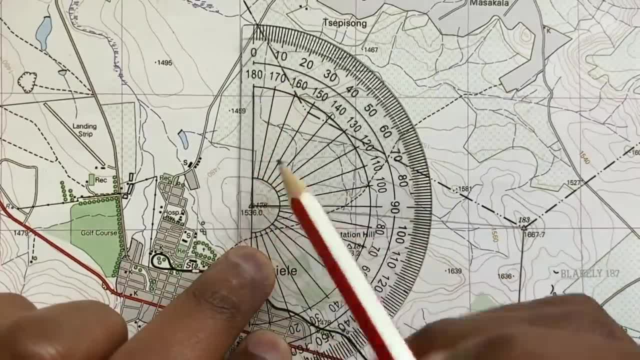 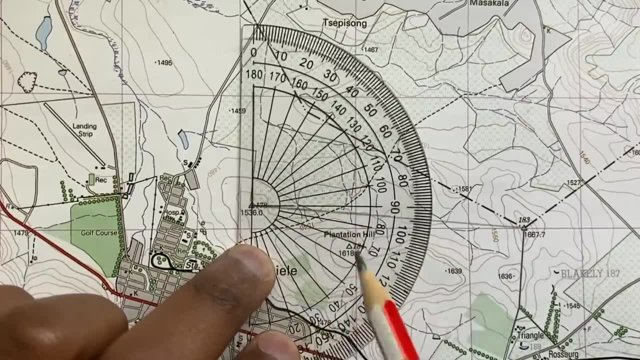 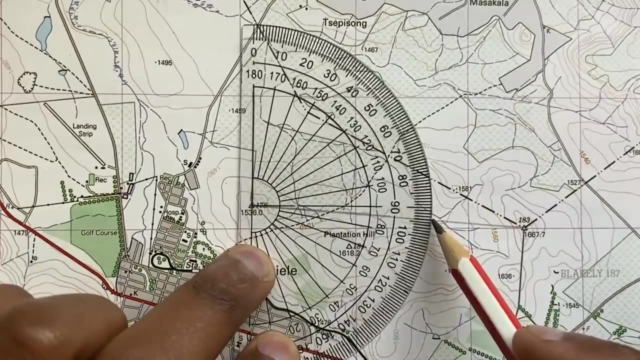 Parallel or adjoined to this line over here, and then you can just measure Your true, Your true bearing. So what I'm getting here, this is 90. This is 91, 92, 93 and 94.. So what I'm getting is: 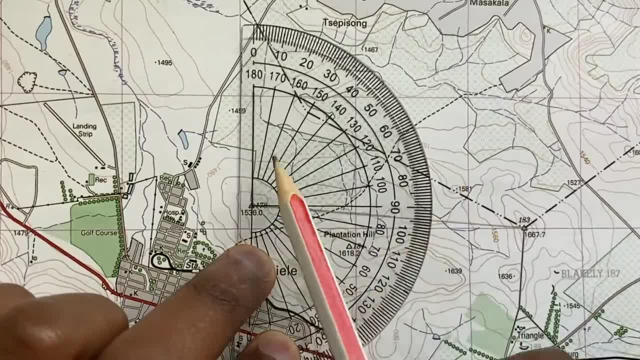 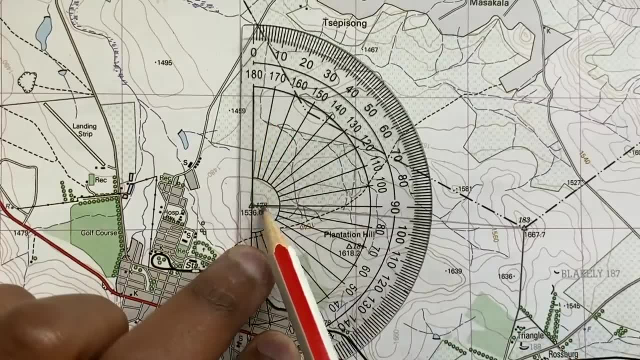 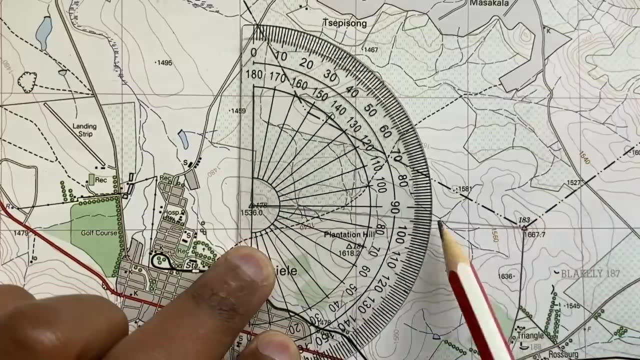 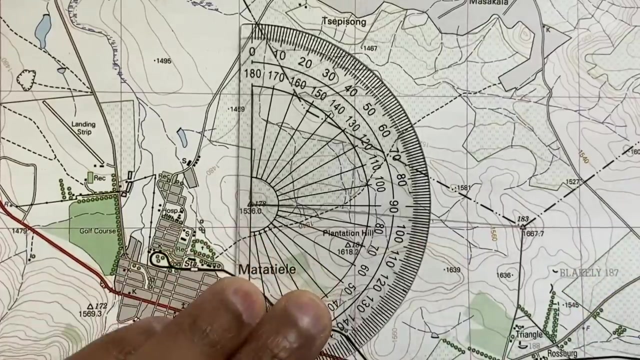 94 to be accurate. So my trick true note or true bearing, rather, from Trickbacon 178 to trickbacon, Trickbacon 183, it's 90, 94 degrees. So it is important to note that you're going to count right at the zero o'clock over here. 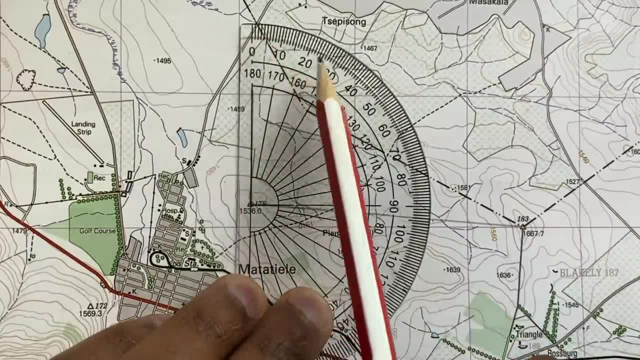 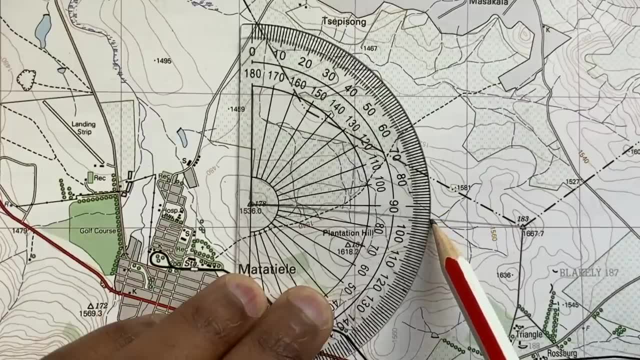 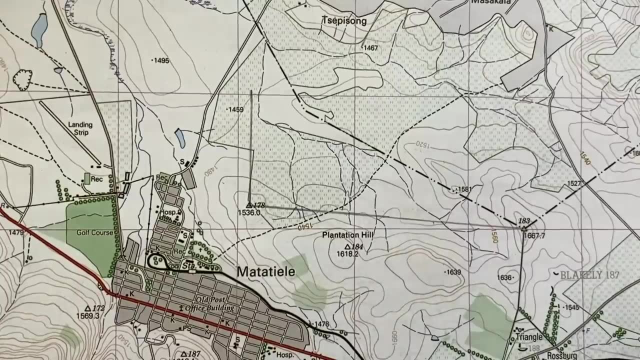 So So it's 10, 20, 30, 40 up until 90, and then you just add whatever that after 90. so I got 90, 94 degrees. So let's reverse the question: what if you were asked to calculate or to find the true? 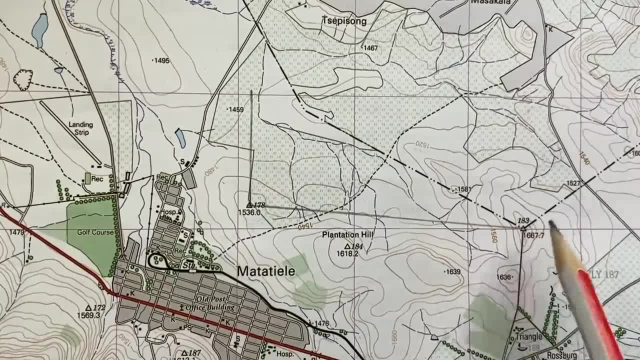 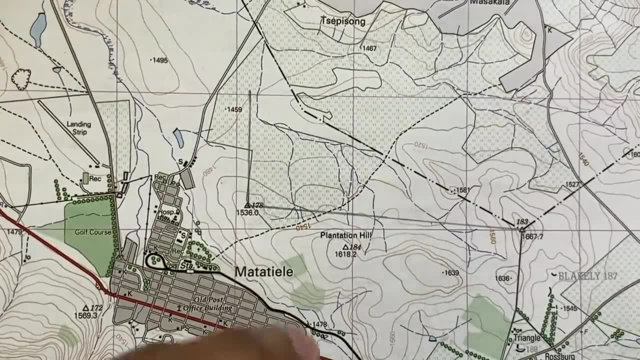 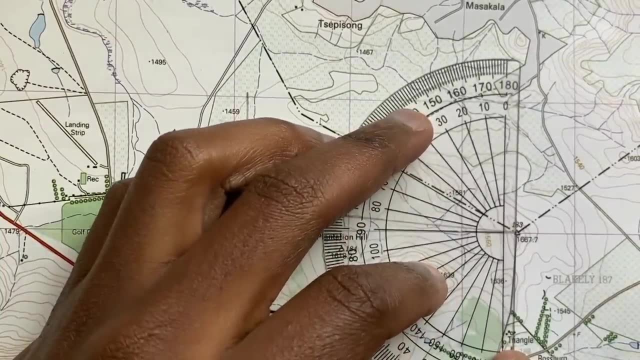 bearing from 183 trickbacon over here to there at 178 trickbacon, we still do the same thing. So the first thing Remember is to try your true. Where do you need to start? which is your from? so I'm going to draw my true North over. 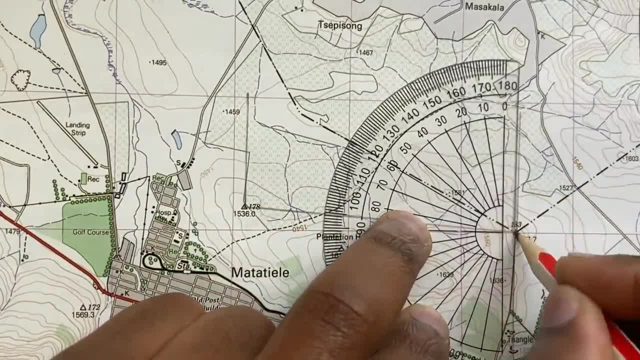 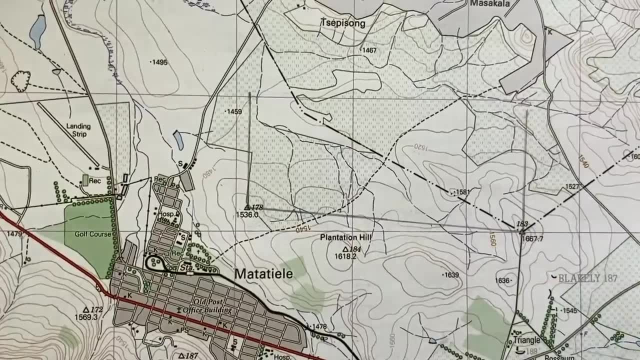 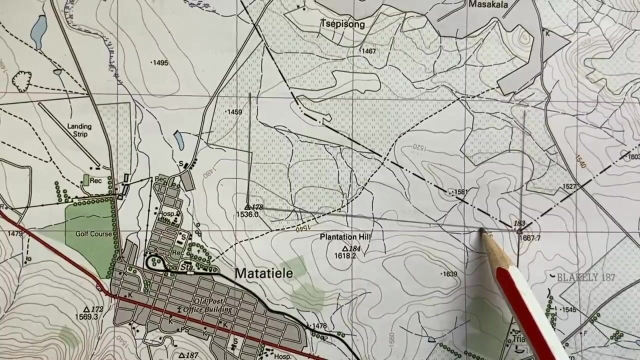 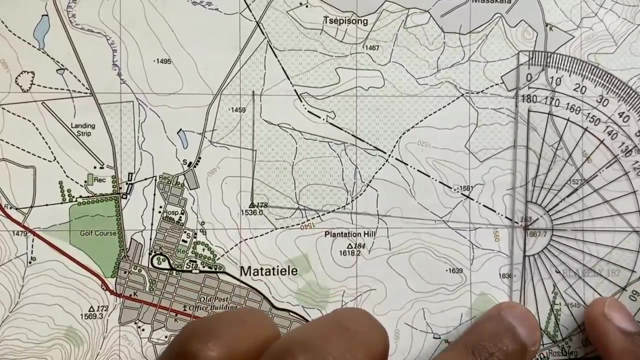 here, which is from 183 and already these lines are already joined. So from here, how I measure my true bearing is still the same way or the same method as I did before, from this true, true north over here, clockwise up until this adjoining line over here. so let's, let's do it so we all know that if I put my ruler over here, 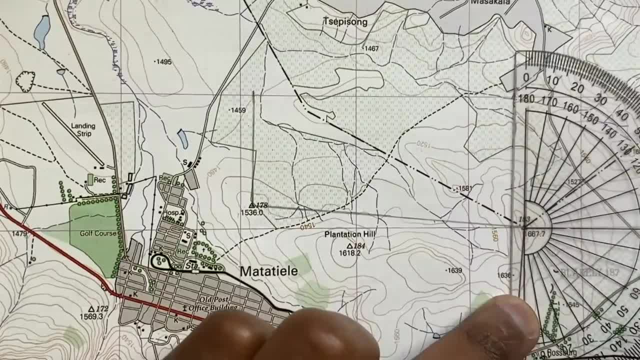 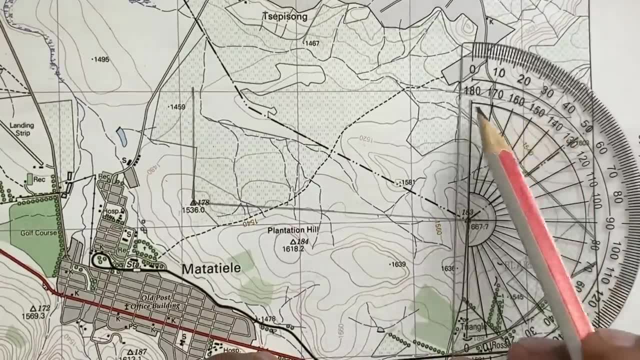 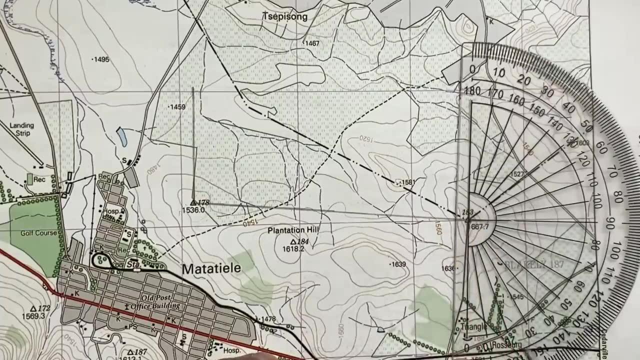 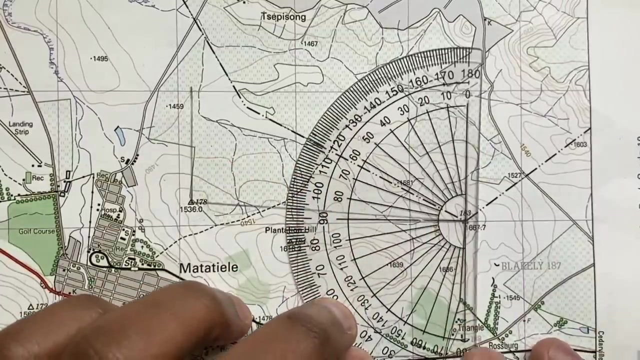 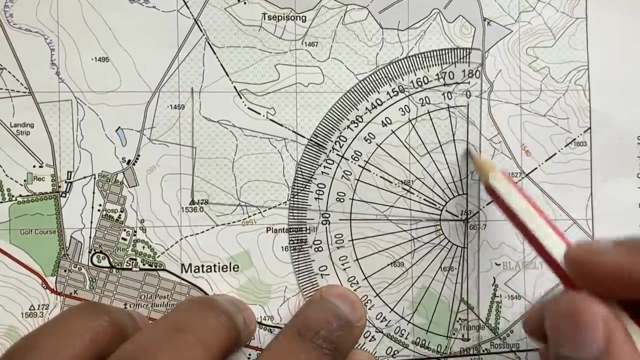 inside this: this is hundred and eighty, this is hundred and hundred and eighty, so this will be 180 plus the angle. whatever angle I'm gonna measure over here. so I know I have 180 plus. now I'm gonna measure the side and I still do the same thing: align my triangle to the inside of the trick bacon and this line: 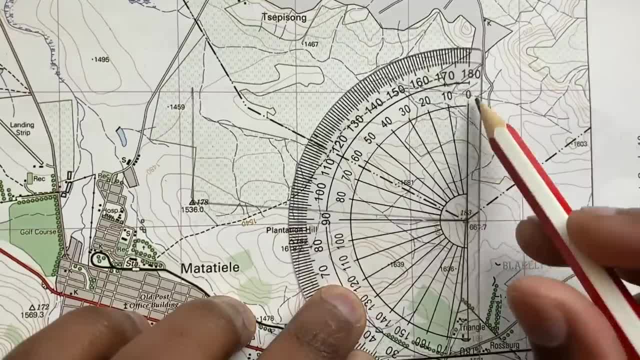 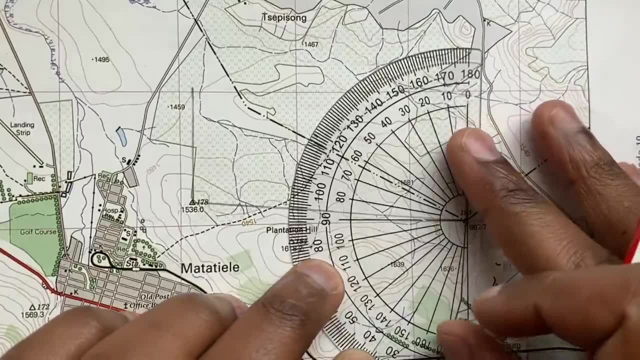 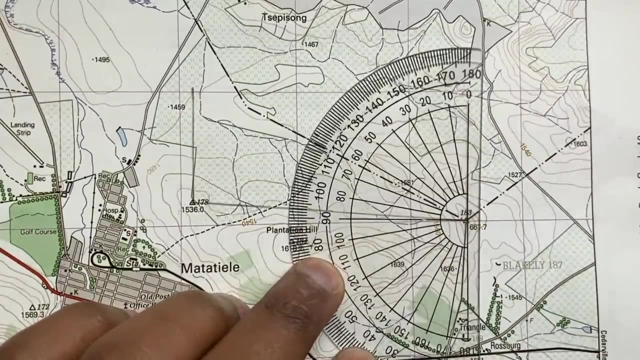 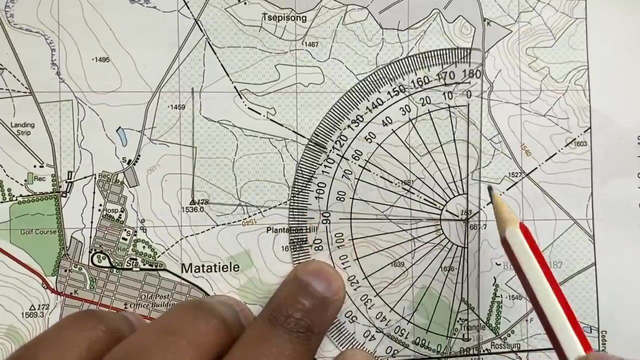 I need to be right on my true north over there and I still get 90. this is 0, up until 90. this is 19, this is 94, so to I mean hundred and eighty, which is that angle plus 90 plus 94 will. 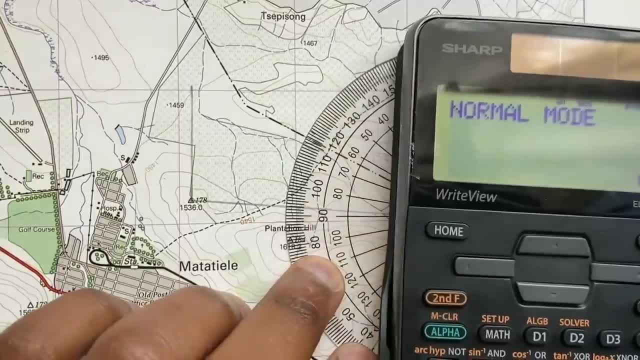 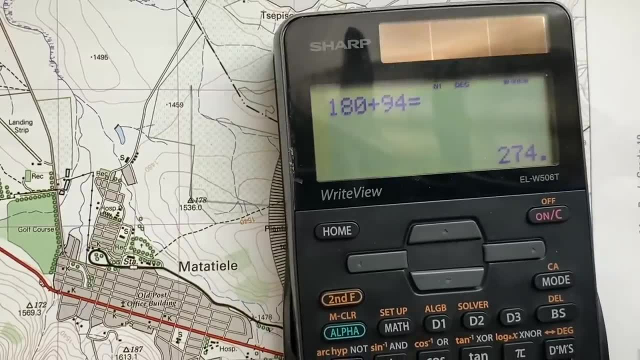 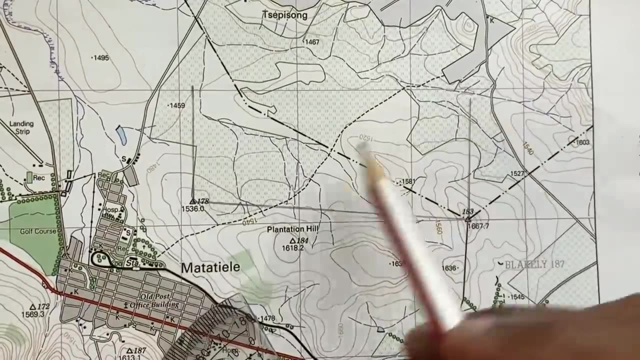 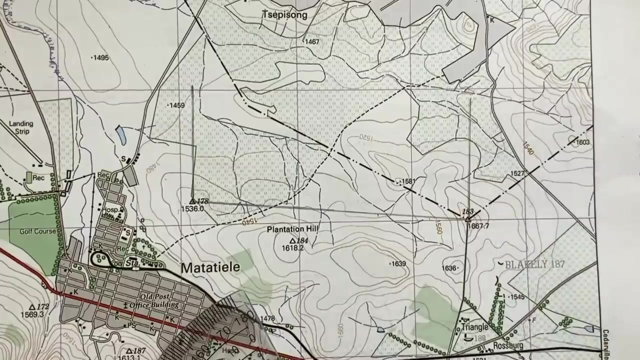 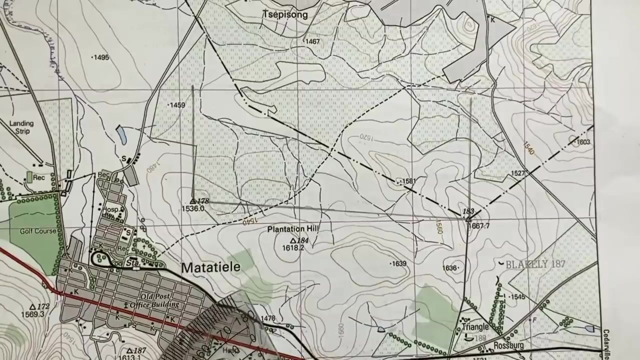 give me two hundred and eighty plus 94 will give me two hundred and seventy four degrees. so that's my true bearing from this trick bacon over here to that one over there. so let's try to calculate magnetic bearing from what we have found, from the first one, which was: 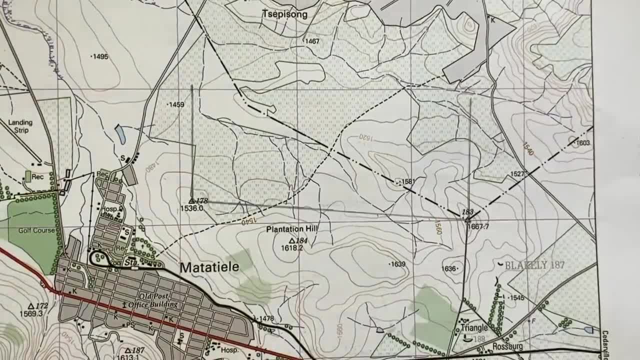 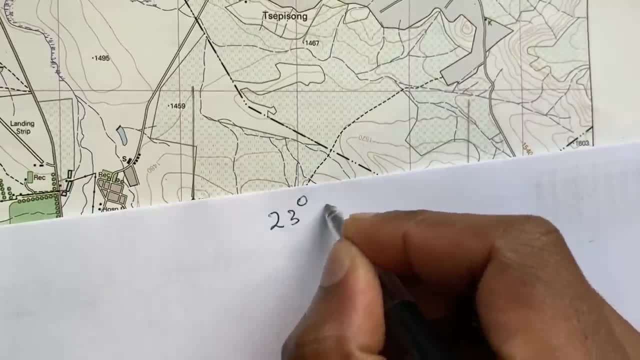 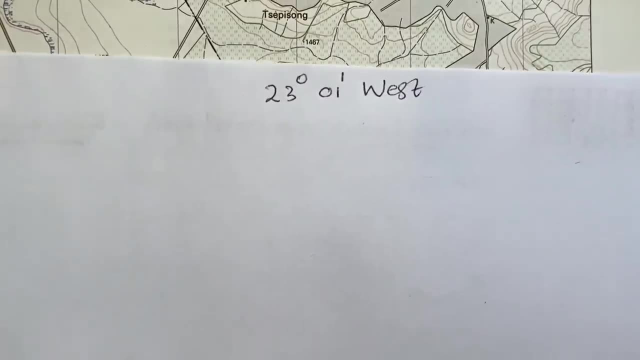 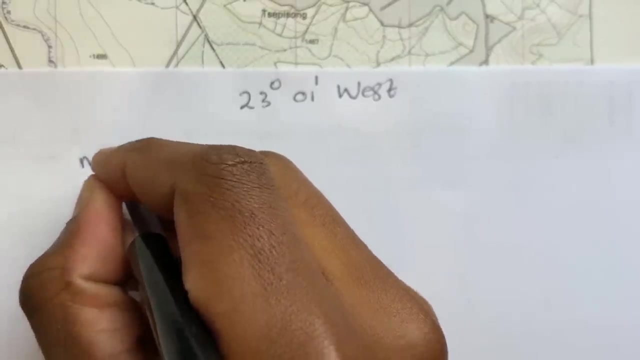 94, 94, oh, oh so the mean magnetic musstress, oh so the mean magnetic rustic intention of this map I'm using is Si 300, 21 minutes west was. so in calculating the magnetic bearing, the formula is 23 degrees, 01 minutes west watts. so in calculating their magnetic bearing the formula is mannantic, very